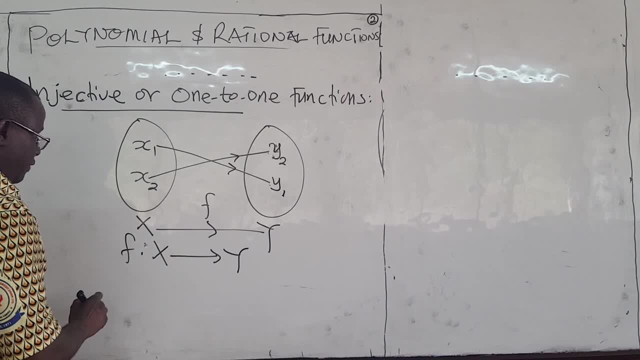 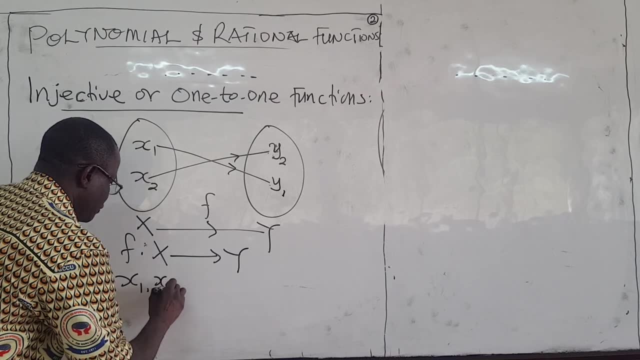 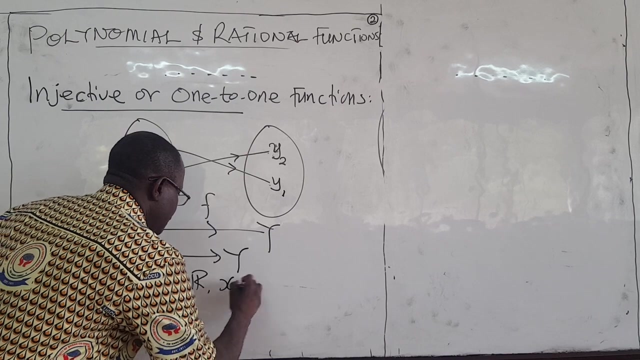 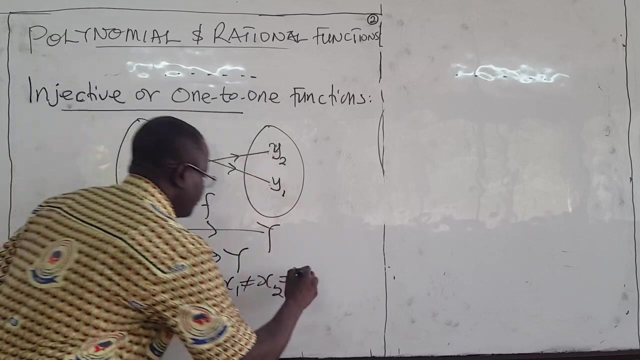 We say that F is one-to-one. if these guys are separate, You have two separate elements: X1, X2.. Right, not left. They are not equal. They are real X1 not equal to X2.. As long as they are separate, you expect that their functional values will be different as well. 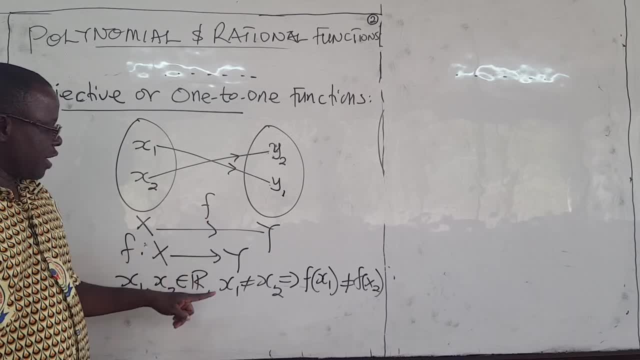 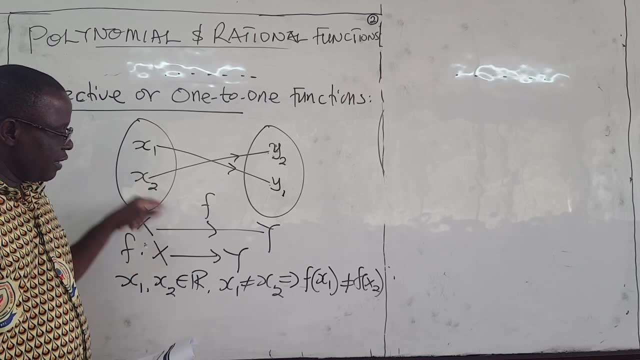 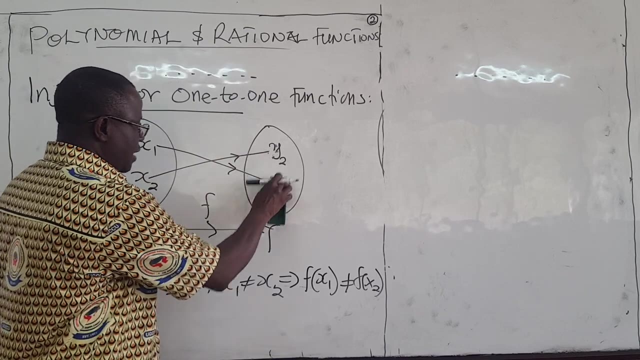 Okay, so that is the formal definition of a function being one-to-one. If these two elements in the set big Y, big X, sorry, if these are separate or different, then their functional values, their values they take on here. Remember that the value that X1 takes here can also be represented by F of X1, right? 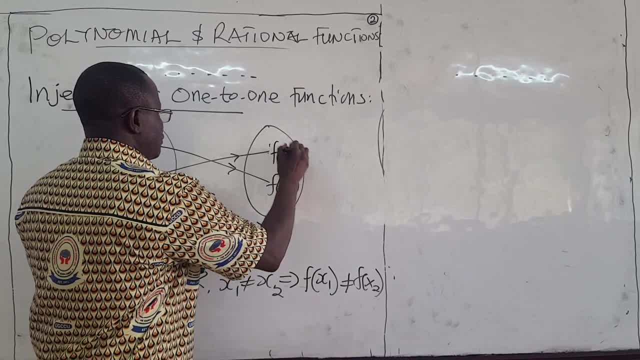 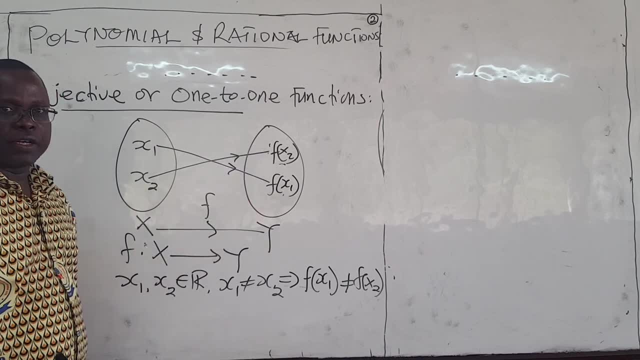 And this is F of X2.. If these are separate, let's take that it should be different as well. If that happens, then the function F is one-to-one. On the other hand, you can also think about it this way: 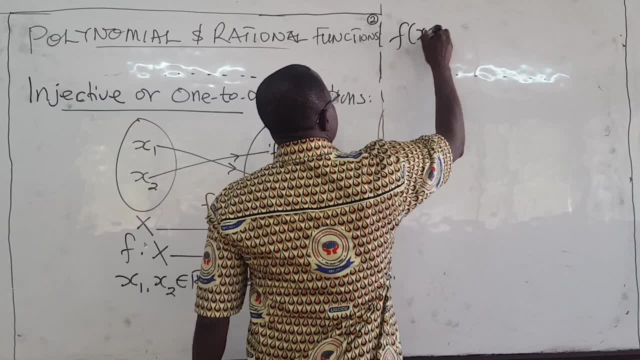 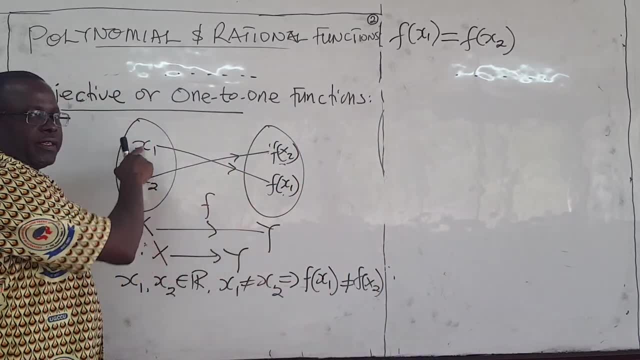 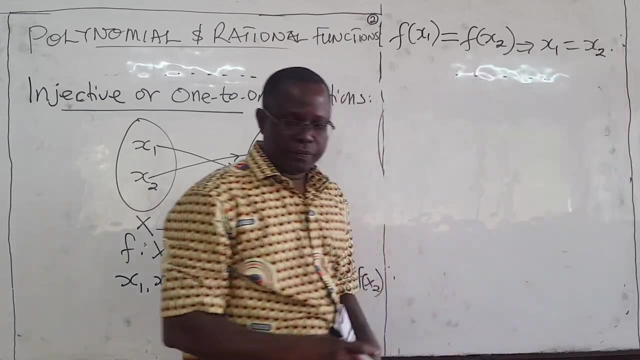 If F of X1 is one-to-one, F of X1 is equal to F of X2.. If they are equal, then this must be equal. Then X1 has to be equal to X2.. Okay, so that is all we mean by a function being one-to-one. 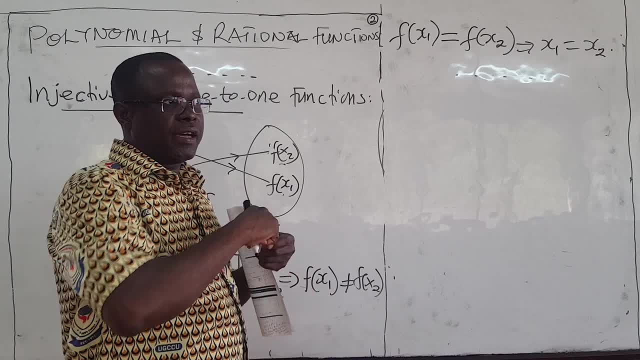 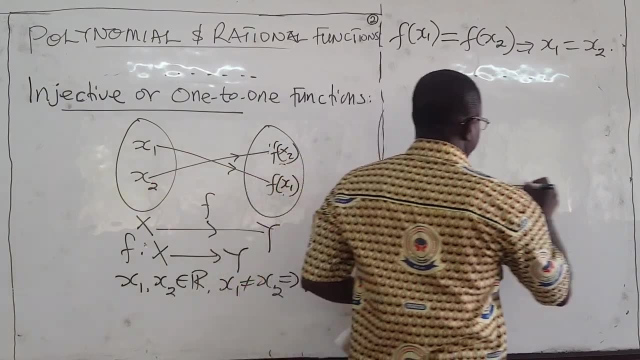 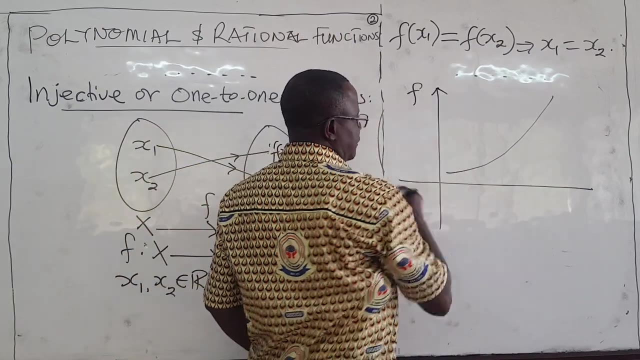 Graphically, one-to-one functions are functions that are either increasing or they are decreasing. Okay, so let's take an example of an increasing function. Suppose that this function is increasing this way: straight line or curve. This is F, that is X. 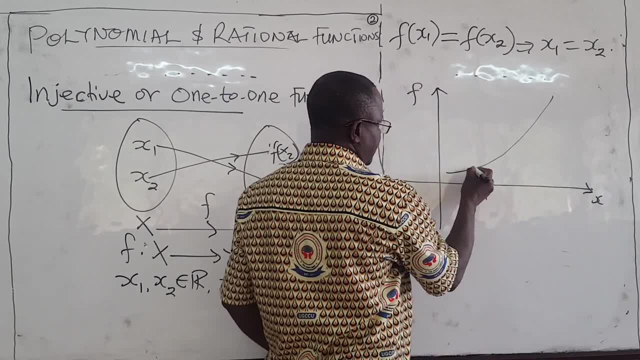 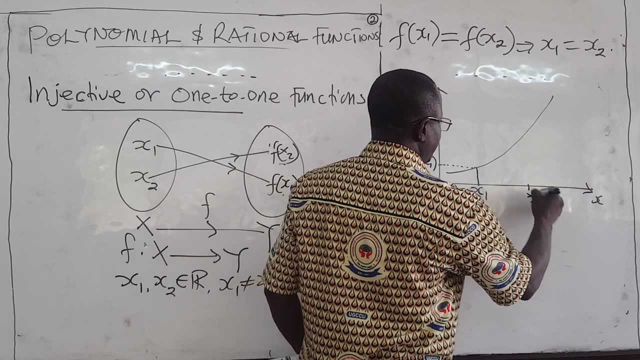 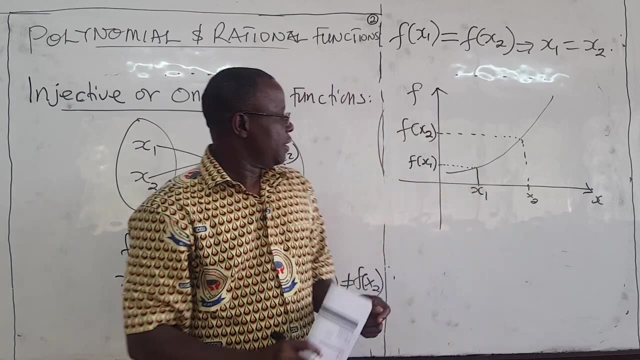 Given X1, here, the value of the function is going to be F of X1, right? And suppose that I have X2 here, It's going to give me F of X2.. Okay, So as long as these two elements are not the same, these guys should be different. 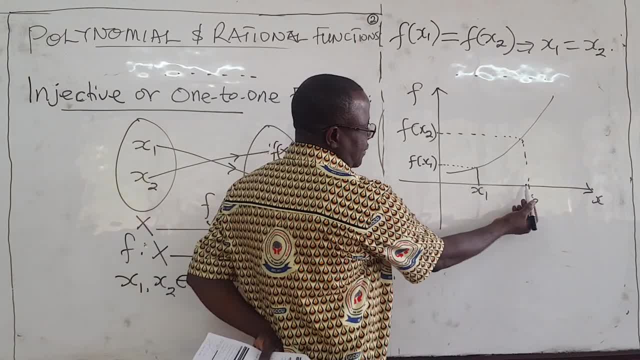 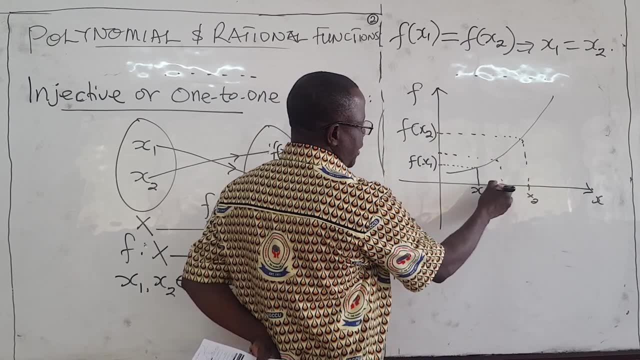 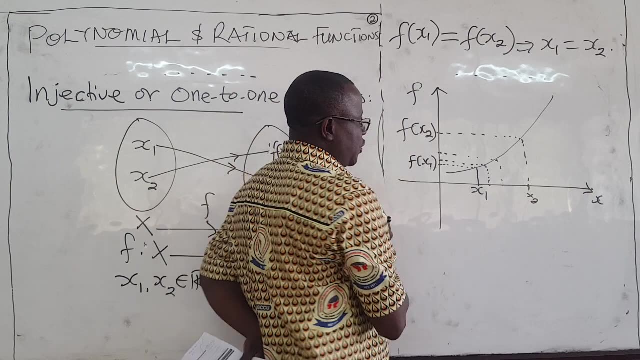 That is the case. F is one-to-one, And you can imagine that as this gets closer to this, suppose X2 moves here, then F2 will have to move here. If it moves here, then this has to move here. If X2 becomes X1, then F of X2 must be equal to F of X1.. 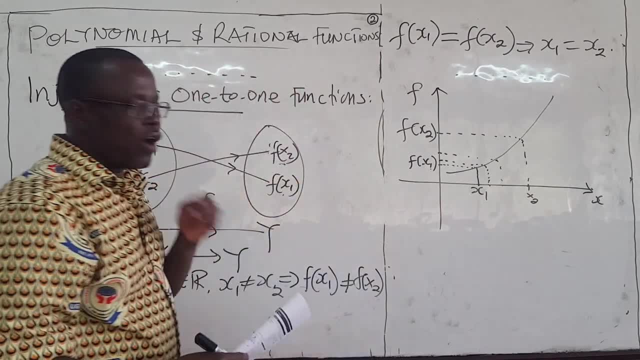 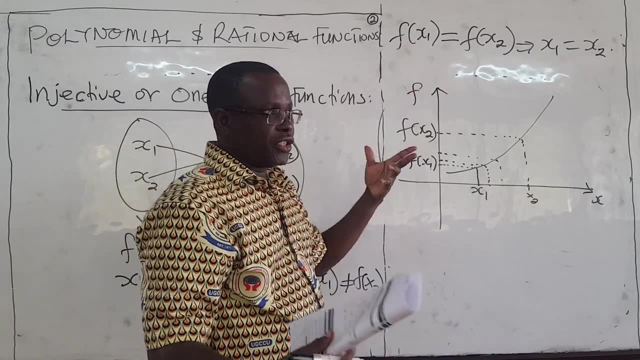 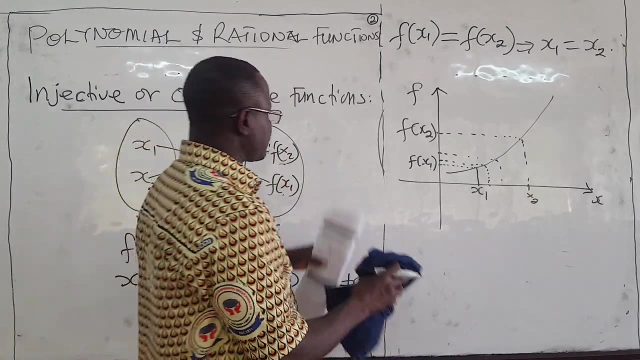 Okay, And so that is that definition. So oftentimes you can either use this definition of the one-to-one function or this one to determine: given a function, to determine whether that function is one-to-one or not. Okay, So we'll look at a couple of examples. 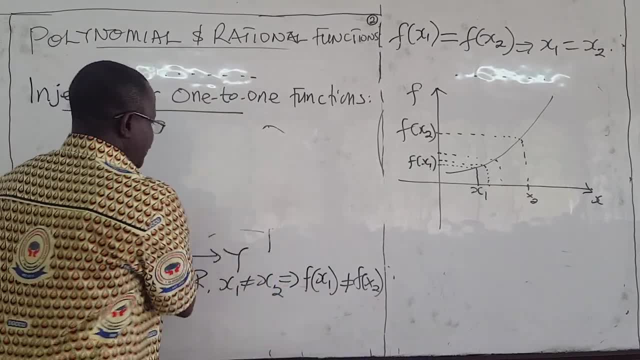 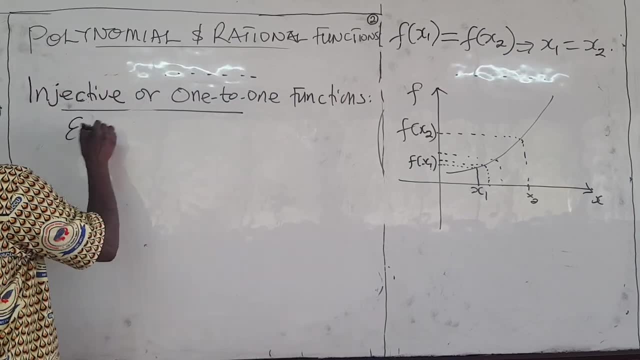 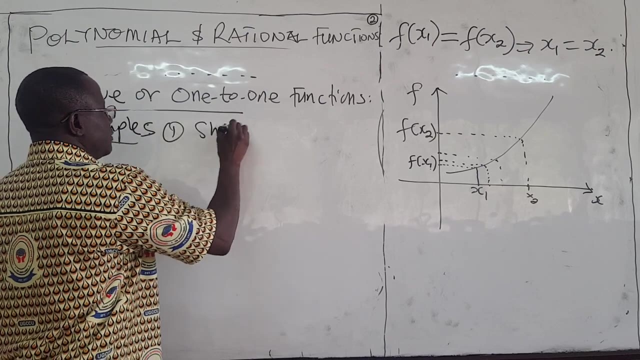 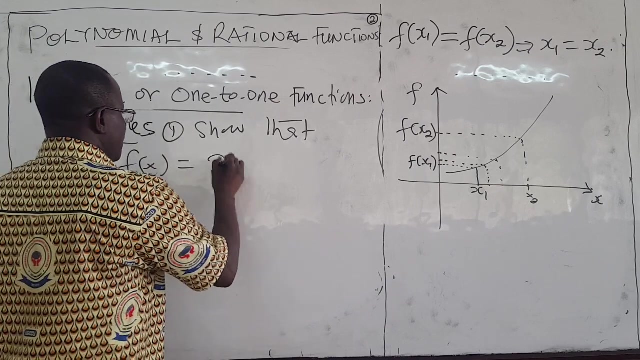 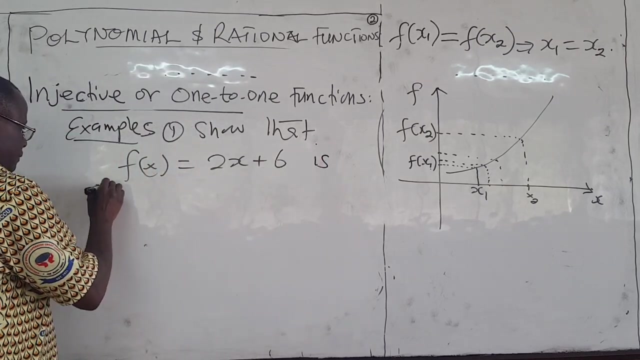 Let's look at a few of these. Okay, So suppose you want to show examples. So examples, Let's say 1 shows that the function F of X, let's say 2X plus what about 6, shows that this is the injector or one-to-one. 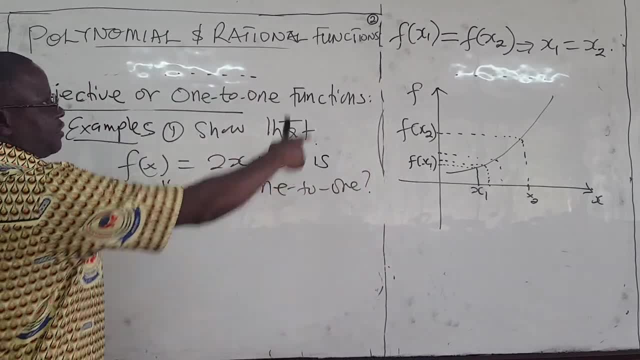 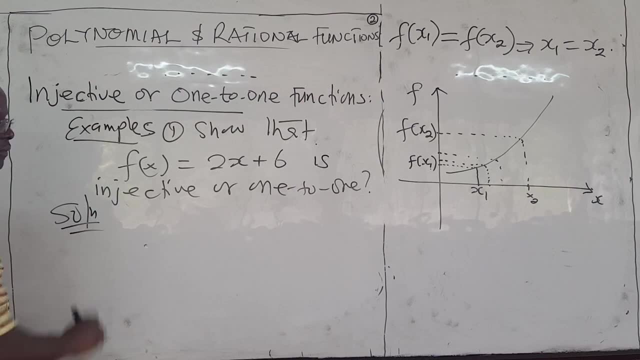 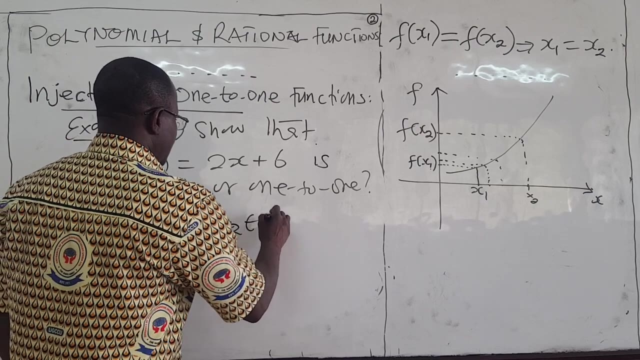 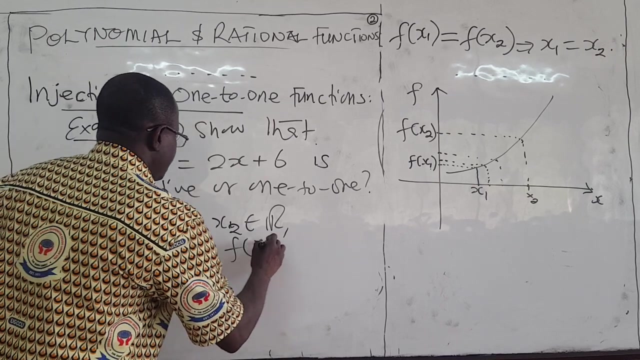 How do you do that? Well, you can use one of the definitions. So let's start with X. This is usually easier, more intuitive to apply. So the solution: So let's X1 and X2 be real, Then F of X1 is equal to F of X2 implies that 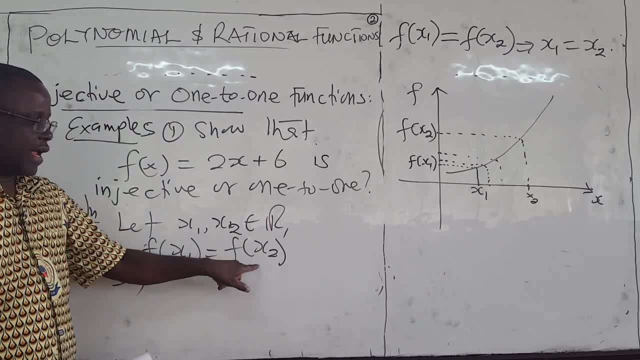 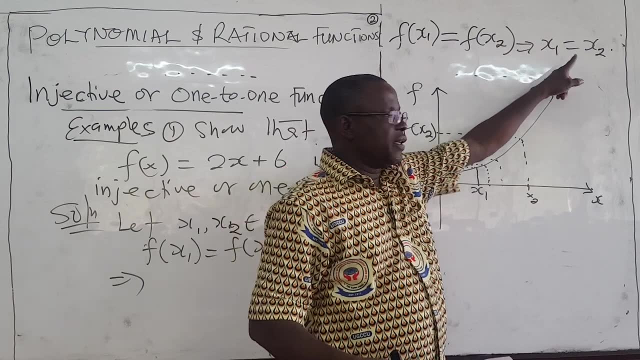 Okay, We want to show that if F of X1 is equal to X2,, we are able to show that X1 is equal to X2, strictly Okay. If we are able to show that, then that proves that the function is one-to-one. 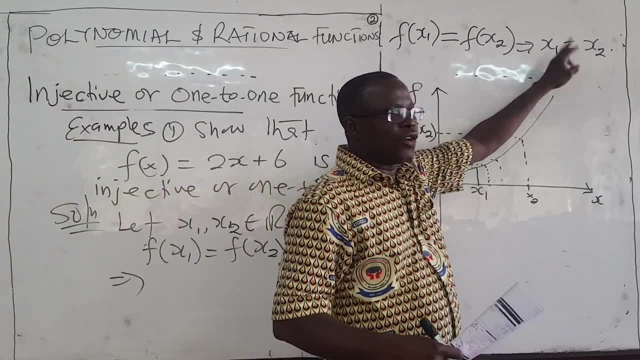 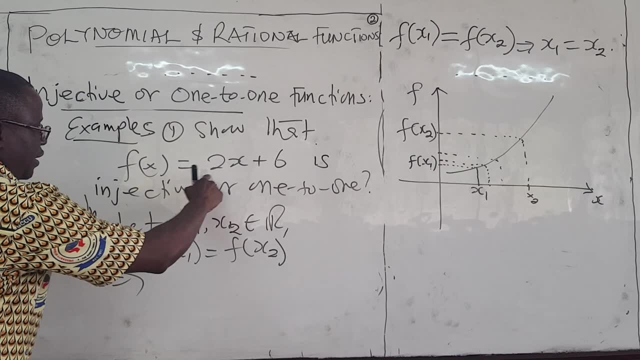 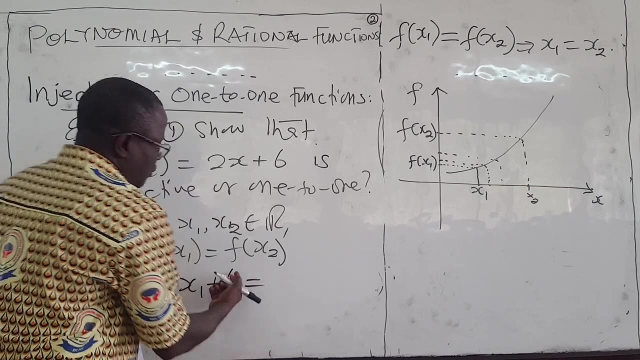 So X1 must be equal to X2 and not anything else. All right, Now F of X1. here I put X1 into here. So wherever I see X, I put in X1. So that is, 2X1 plus 6, is equal to F of X2.. 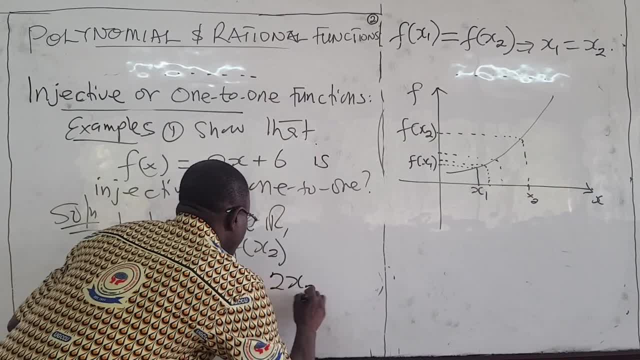 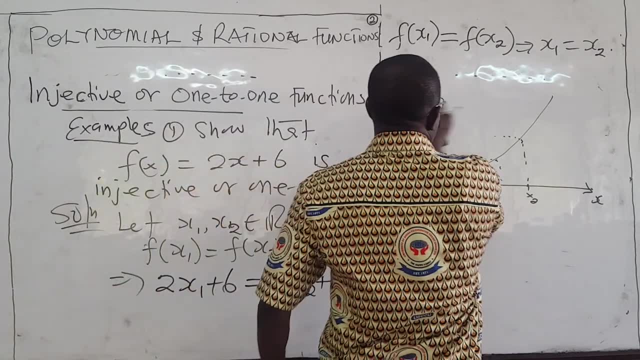 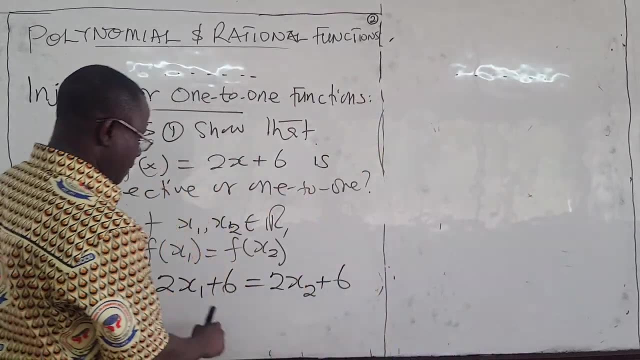 So wherever I see X, I put in X2 plus 6.. Okay, So I have that. That solves this. Let me get rid of that. Okay, So now from here, it's positive 6,, positive 6.. 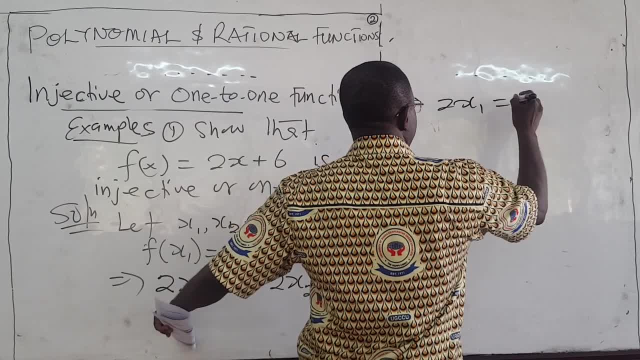 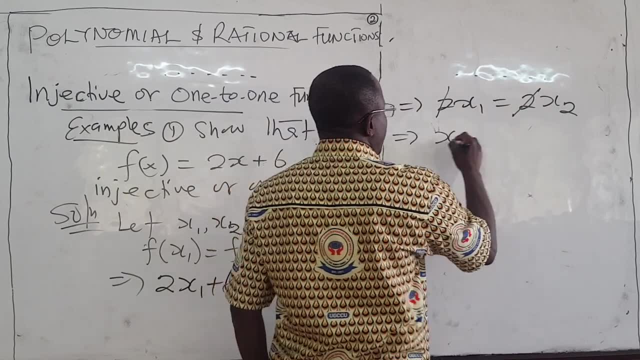 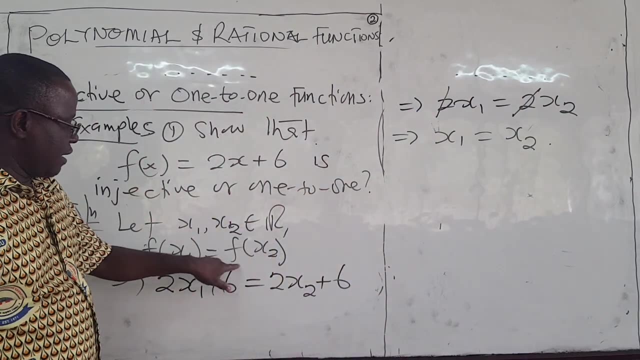 They cancel out, And so I have: 2X1 is equal to X2.. This guy cancels out S, It cancels out S I have. 2X1 is equal to X2.. So if F of X1 is equal to F of X2, we have shown that X1 is equal to X2.. 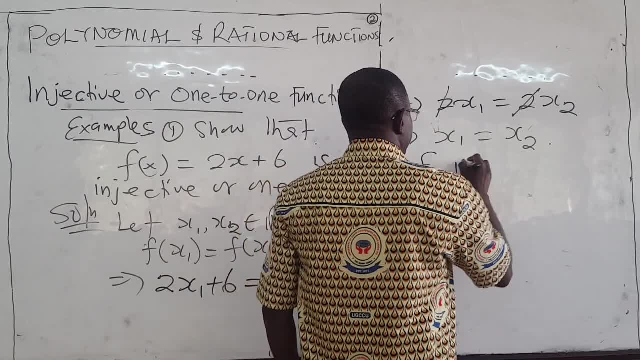 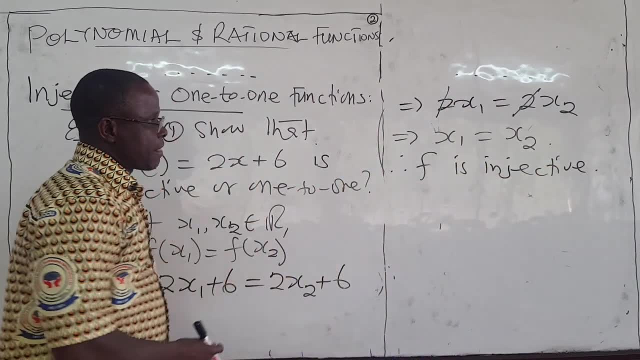 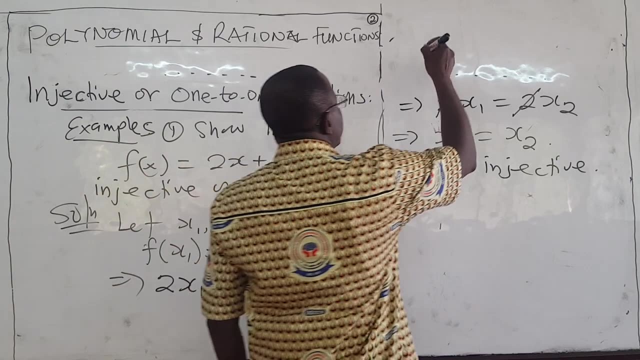 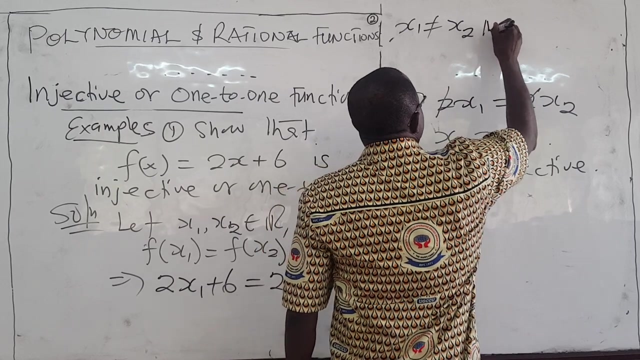 Therefore, the function F is integer 2.. Okay, It's one-to-one. You could have shown this or proved this using the other definition. Remember: the other one says that if x1 is not equal to x2, then f of x1 must not be equal to f of x. 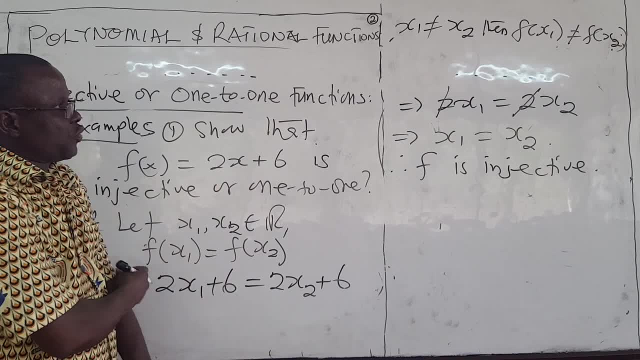 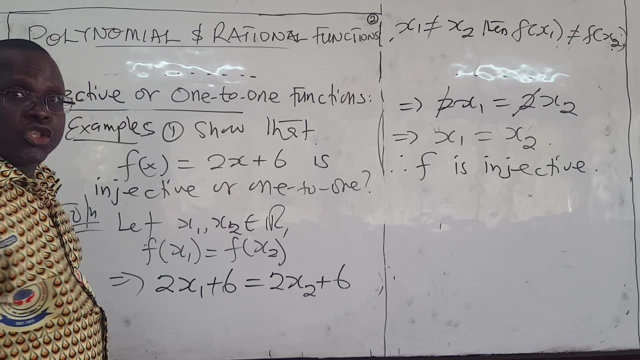 Okay, So you can do a reason-based definition as well. As I said, that is usually not as intuitive, but you can still do it, So what you do in that case. so this is an alternative way of proving that it is 1 to 1.. 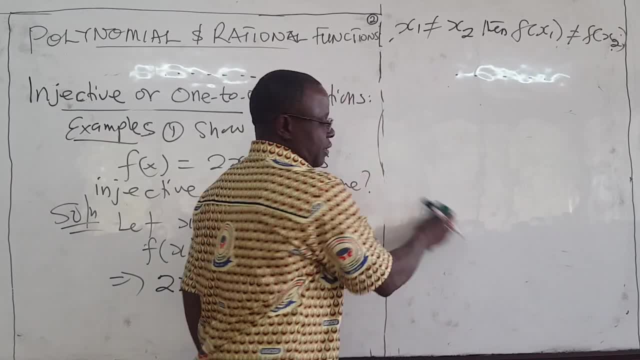 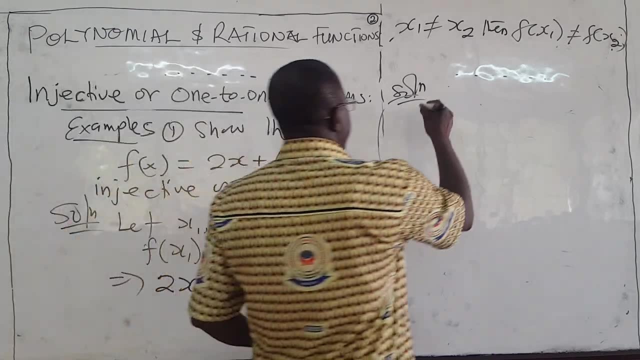 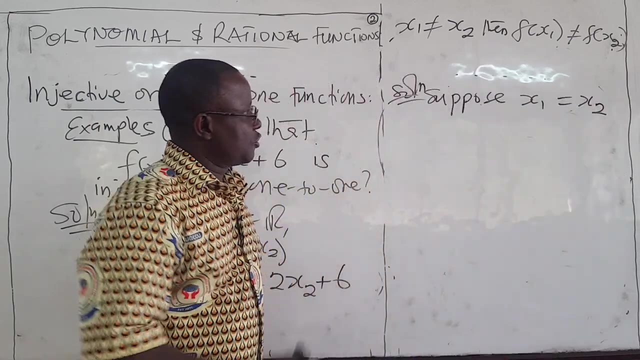 What you do is this: So you do the same thing, you take your x1 and x2, and then let's suppose that x1 is equal to x2.. Sorry, not Okay. So this is not 1 to 1.. 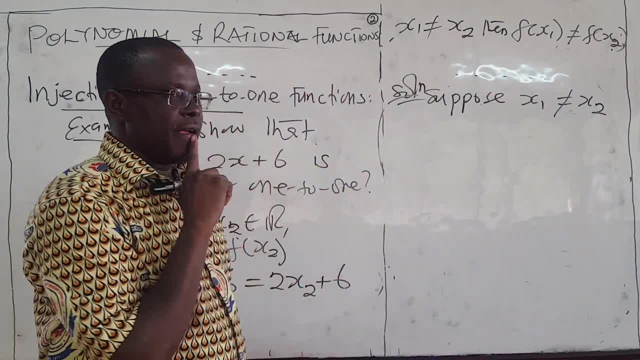 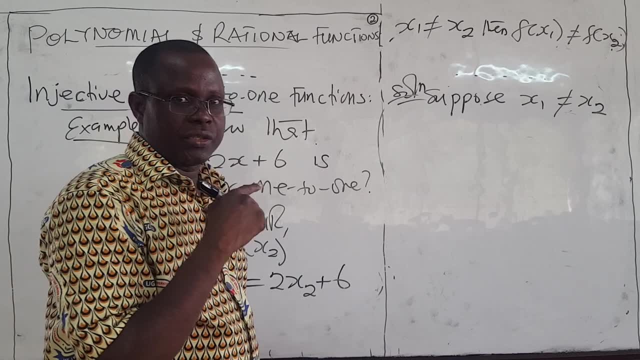 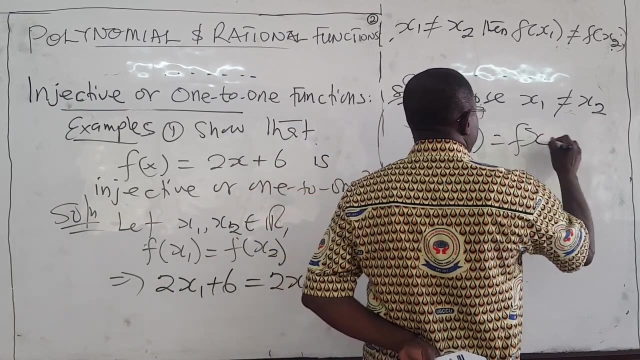 So suppose x1 is not equal to x2.. Okay, So what? we end up showing that f of x1 is not equal to f of x2.. If not, then there's a contradiction, Right? Okay, So now then we go. f of x1 plus f of x2 implies that we've already proved this. 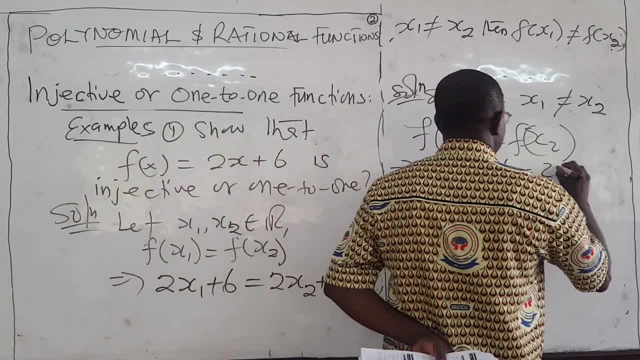 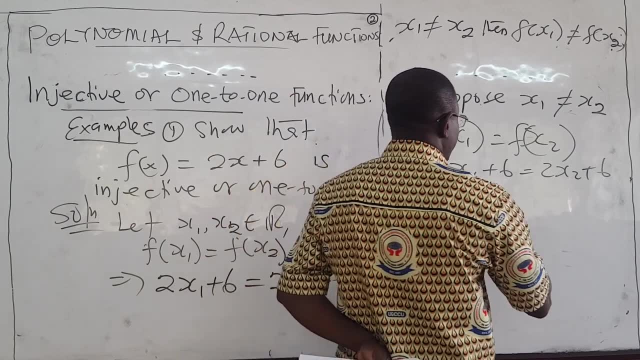 All right From here. 2x1 plus 6 is equal to 2x2 plus 6.. 2 is cancelled out, and if 6 is cancelled out, 2 cancels out and then x1 is equal to x2.. 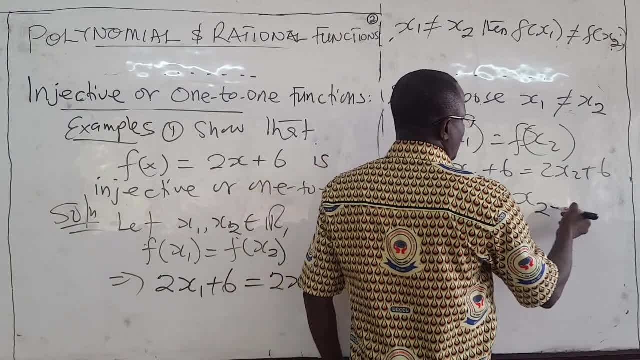 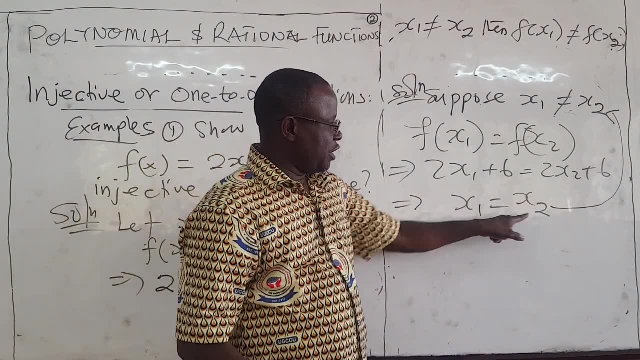 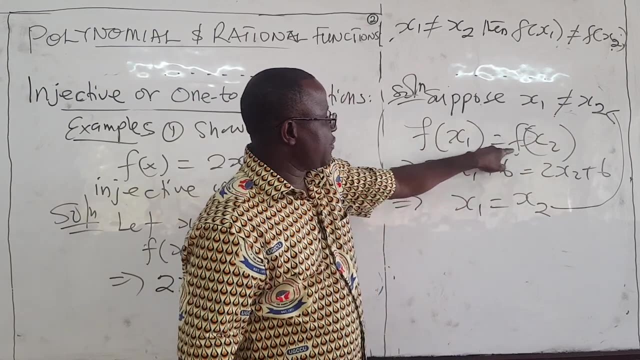 But look, We suppose that x1, here we suppose that x1 should not be equal to x2.. So if we are getting x1 to be equal to x2, that is a contradiction. It's contradicting this, which means that this where we started from. 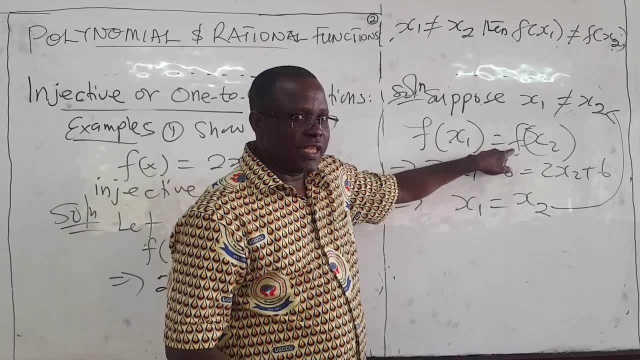 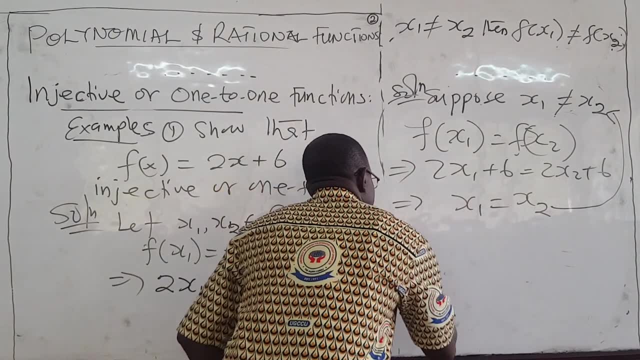 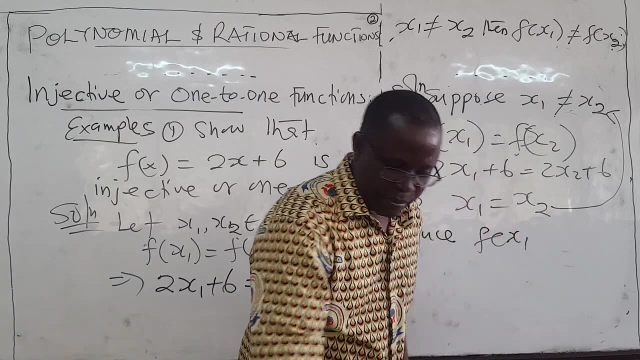 this is not correct. This is wrong, And so this means that f of x1 must not be equal to f of x2.. So this implies that, or you can say that, therefore, f of x1, well, let me, let me see the problem. 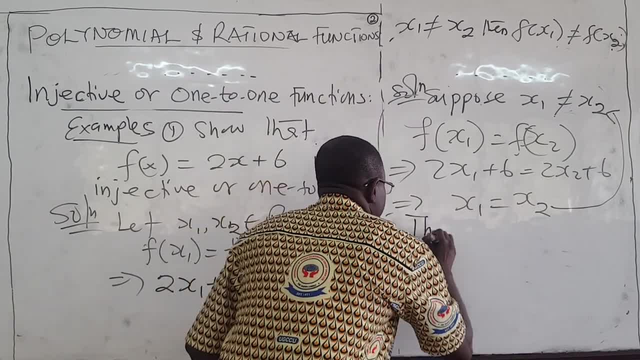 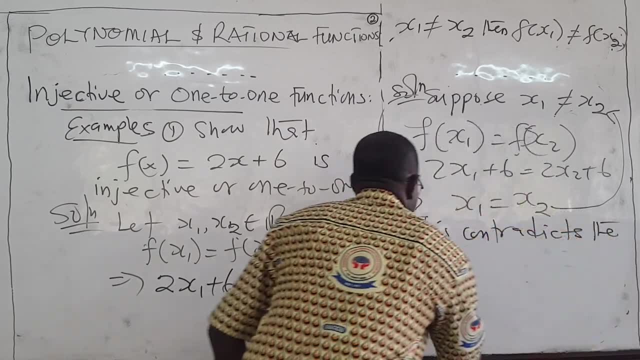 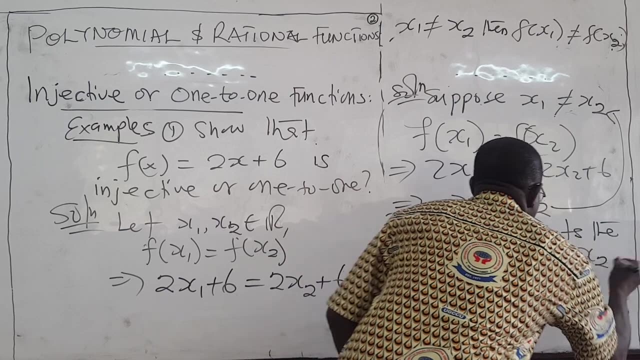 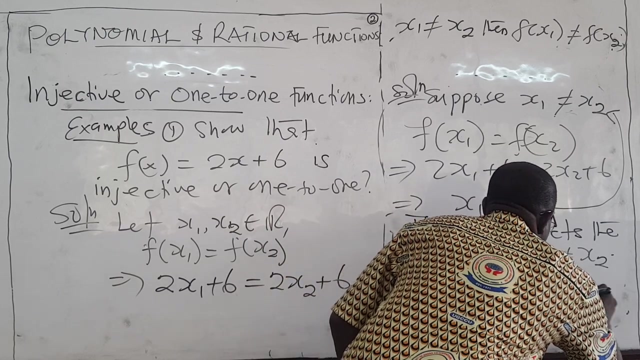 Let me see the problem. So I will say that this contradicts right, contradicts the assumption or the fact that x1 is not equal to x2.. Therefore, f of x1. It's not equal to f of x2.. 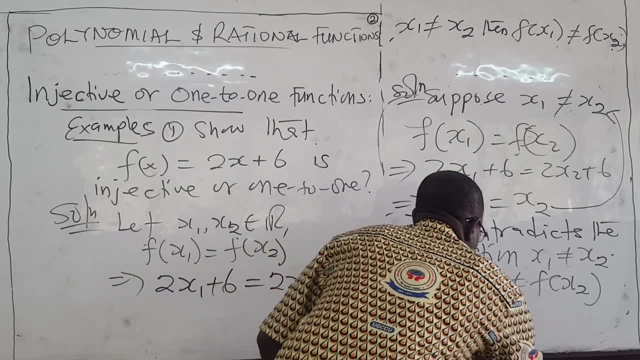 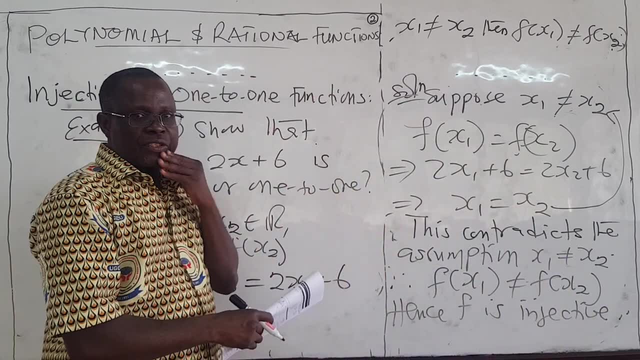 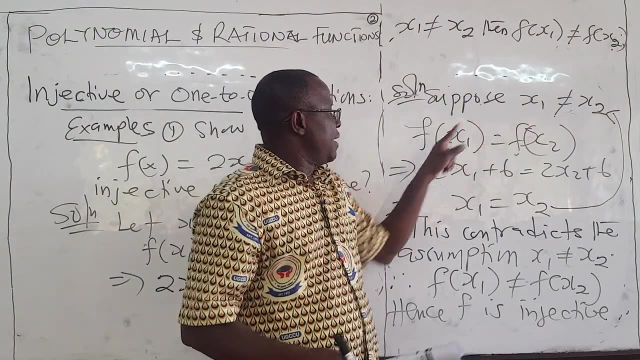 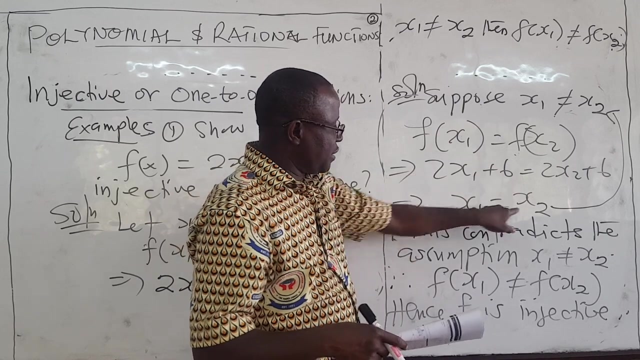 Hence f is a judge, You see. So this is an unalternative way of proving. You start by supposing that x1 is not equal to x2, and then you suppose that this is equal to this. You end up showing that x1 is equal to x2.. 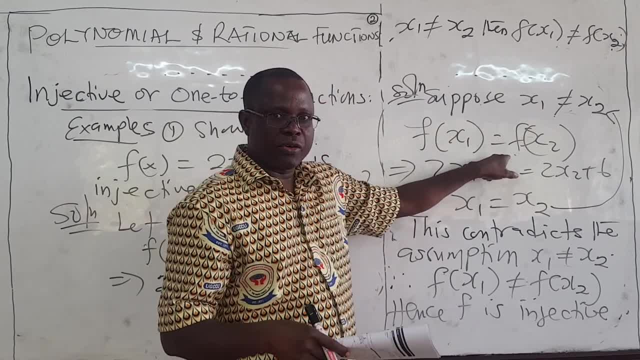 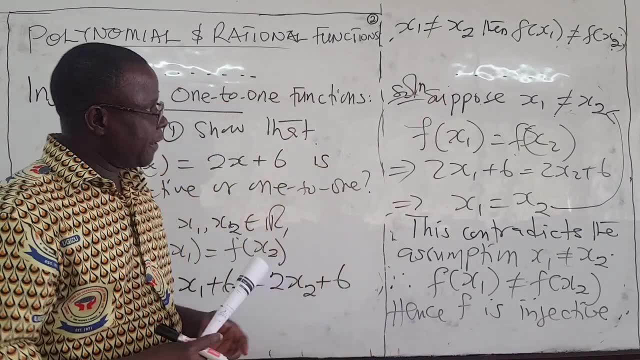 But that is a contradiction, which means that f of x1 must not be equal to f of x2. And that satisfies this. Therefore, f is injective. Okay, All right, Let's move on to a second example. All right, 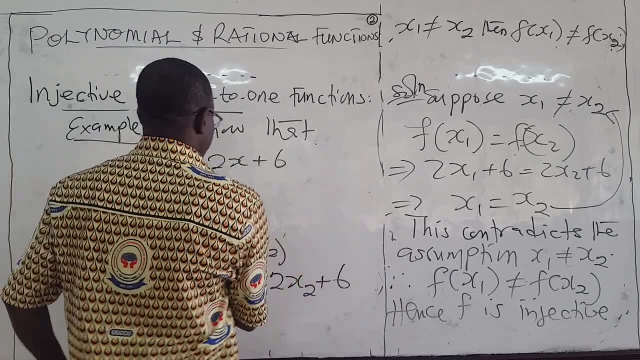 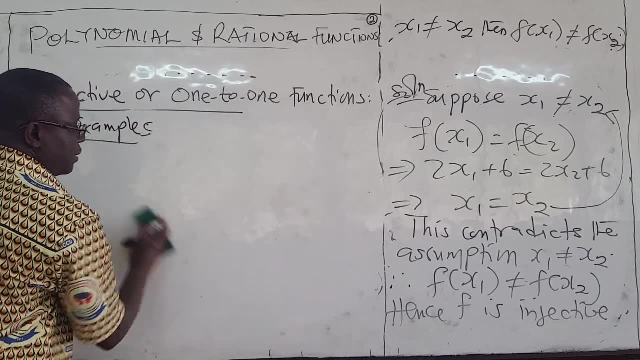 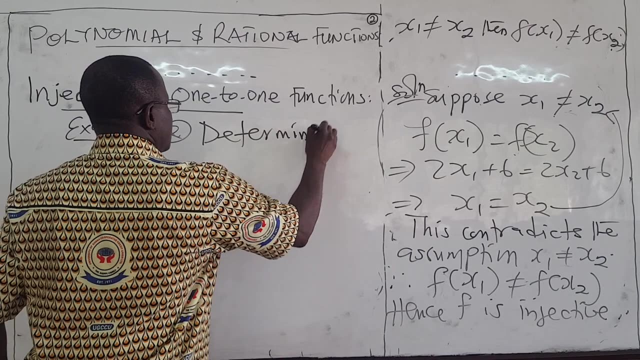 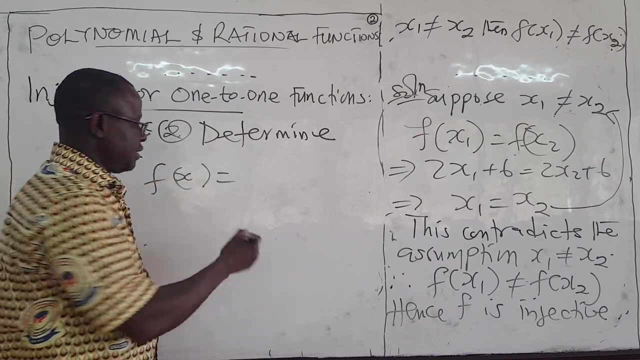 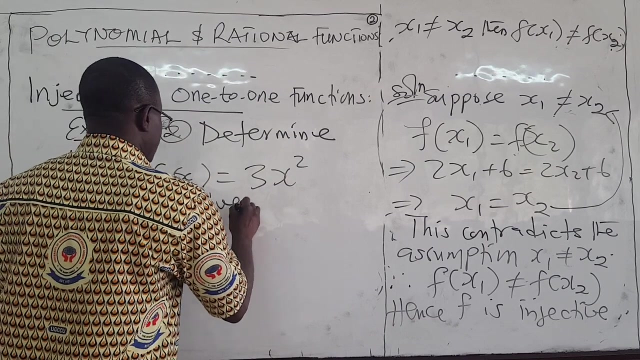 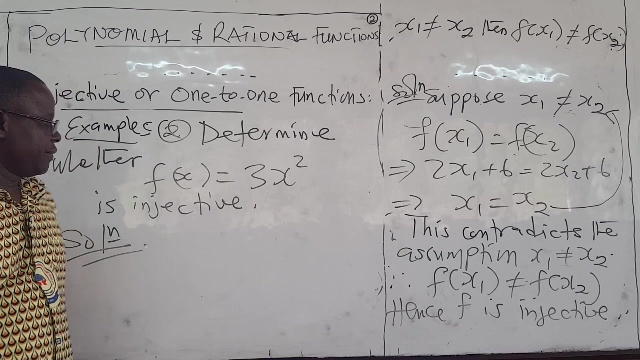 Let's look at one more example here. Determine whether, determine, all right. Example two: determine whether f of x is equal to, let's say, 30: x squared is injective, All right. So what do you do? We do the same thing. 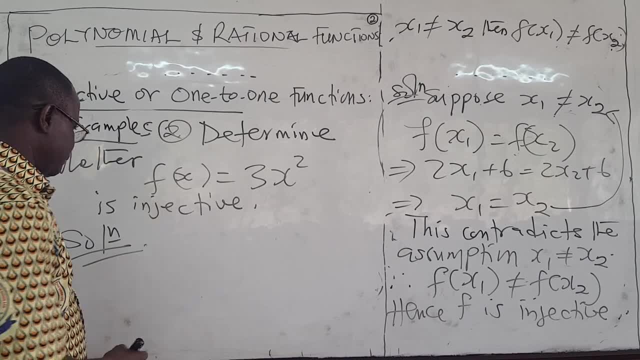 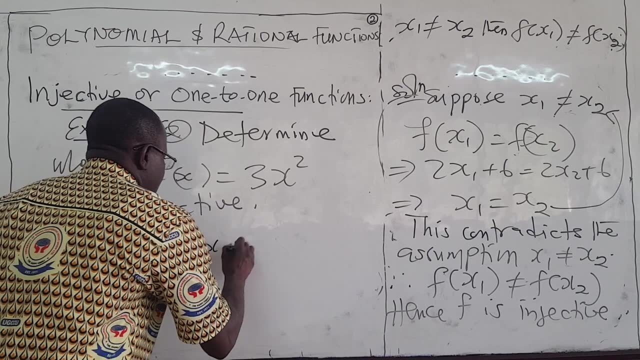 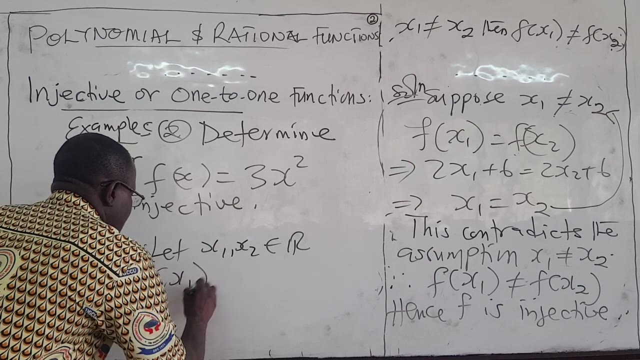 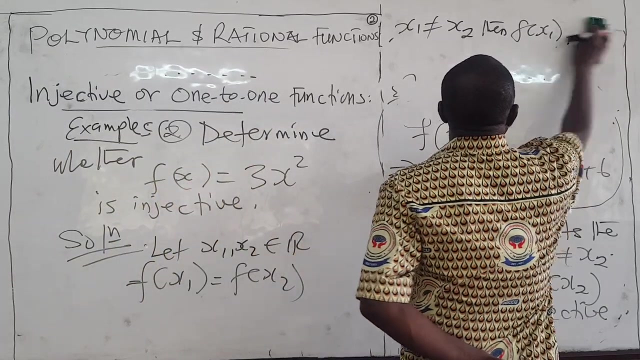 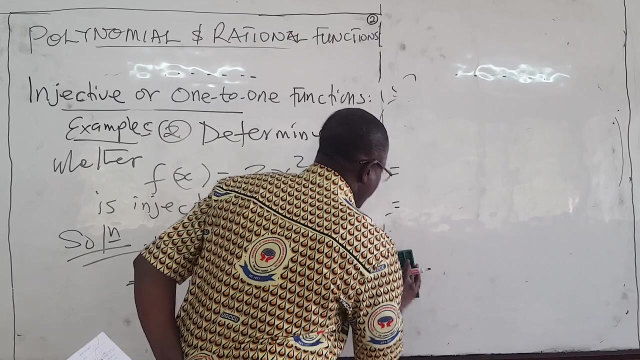 Let's try to see whether it is one-to-one or not. So again you choose x1, x2 real. Then f of x1 is equal to f of x2. implies that implies that. so plug x1 and x2 into there. 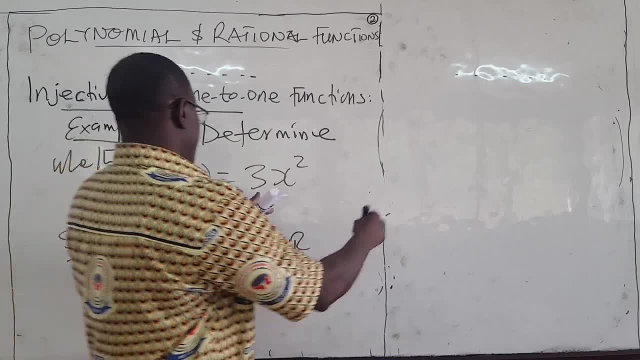 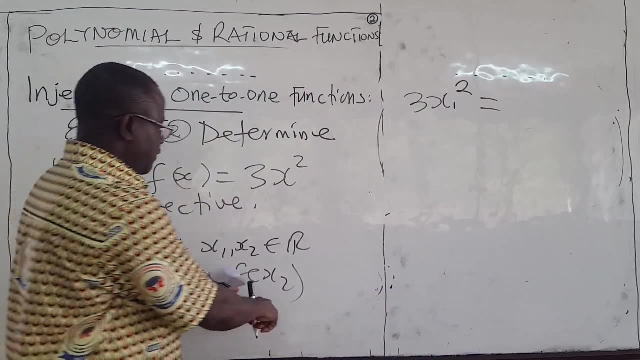 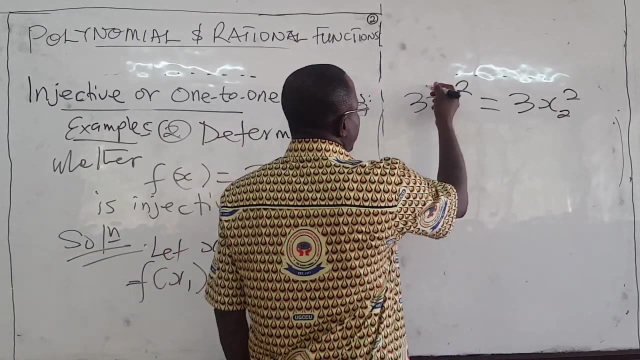 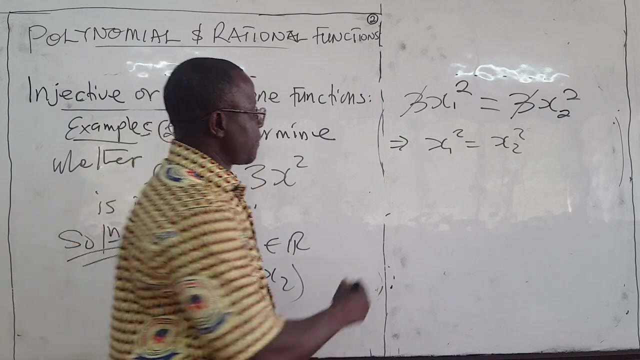 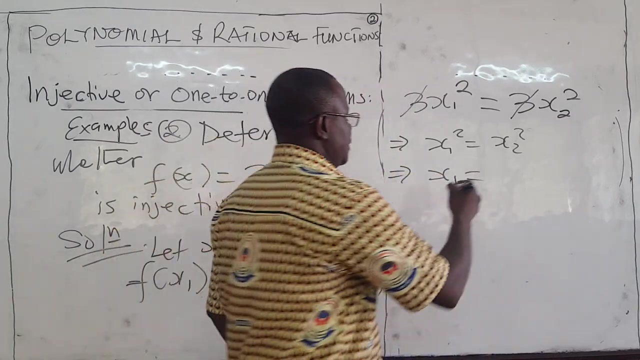 into the equation of the function here. So this implies that 3x1 squared is equal to 3, so that is, f of x1, f of x2 will be 3, x2 squared- right. Okay, now here we have to cancel out, which implies that x1 squared is equal to x2 squared itself of x1 to the square root. so this implies that x1, remember it- is going to be plus or minus, plus or minus the square root of x2 squared. 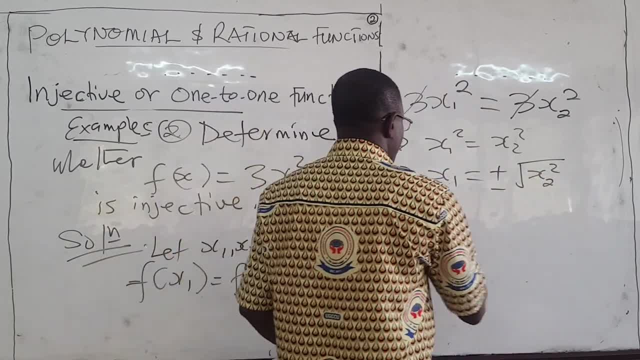 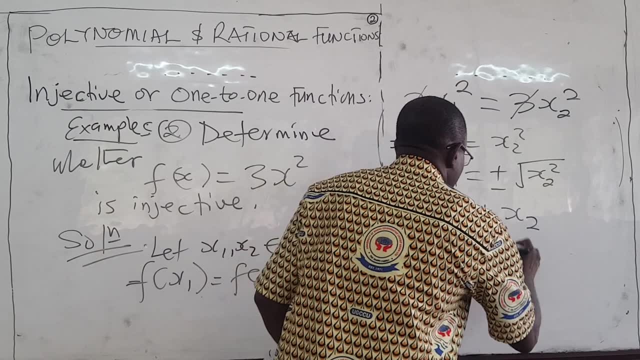 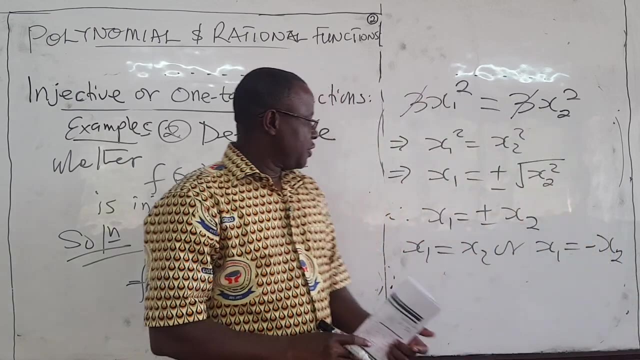 The square root of x2 squared is x2,. therefore x1 is plus or minus x2.. So x1 is equal to x2, or x1 is equal to negative x2. So x1 is not strictly equal to x2.. It. 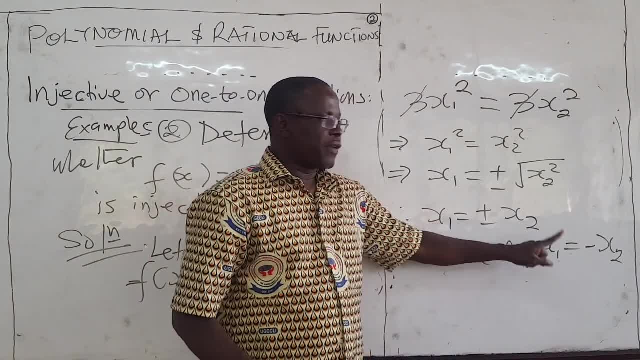 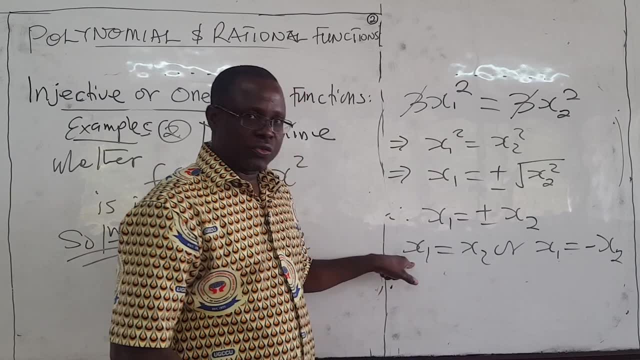 could be this or it could be that, But for it to be 1 to 1, if f of x1 is equal to f of x2, we expect that x1 must strictly be equal to f of x2.. So because of this, we conclude. 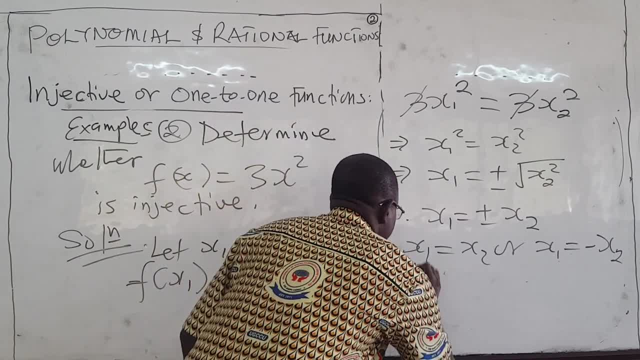 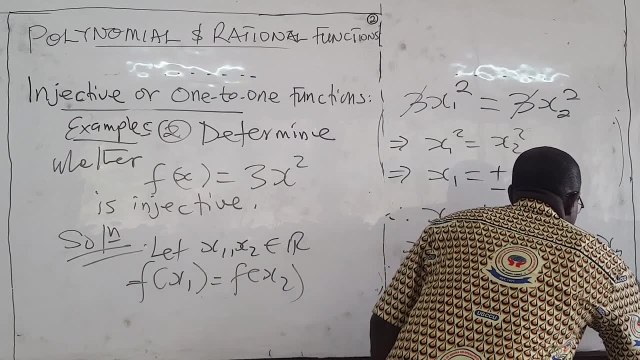 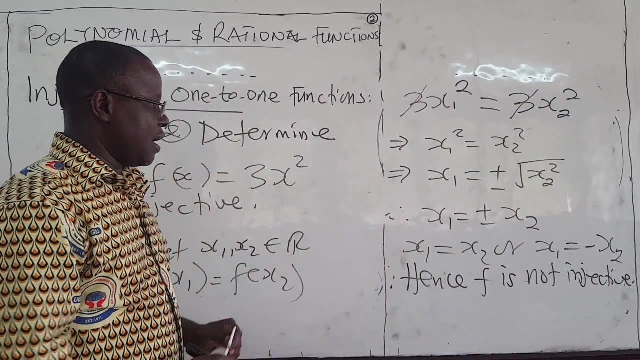 that f is not 1 to 1.. Hence f is not injective or not 1 to 1.. So that is how you prove that a function is 1 to 1 or not. In the next video I'm going to do one on suggestive or onto. functions, So I'll be right back.